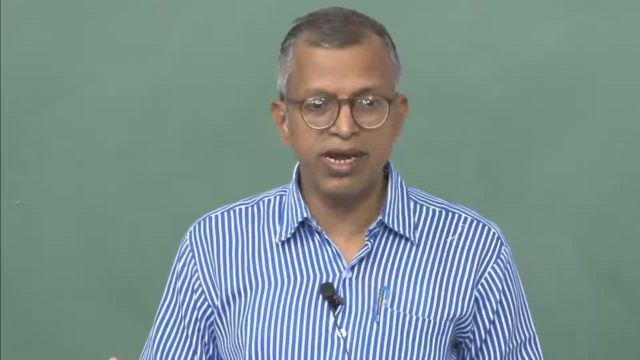 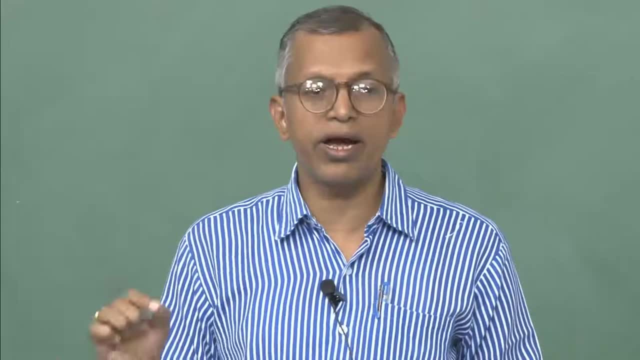 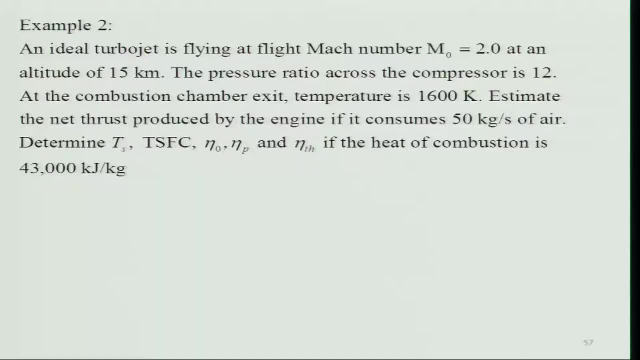 occurring at the maximum specific thrust, And then we looked at propulsive efficiency. What we will do now that we will now take up an example in the turbo jet engine and look at how we can solve a problem, particularly not for carrying out parametric cycle analysis- 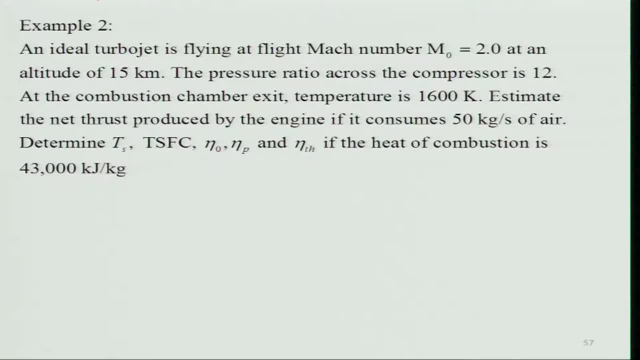 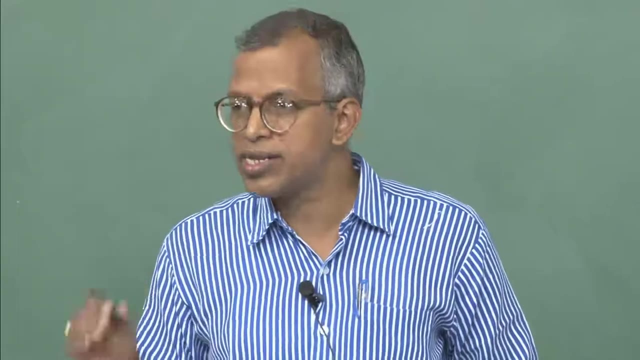 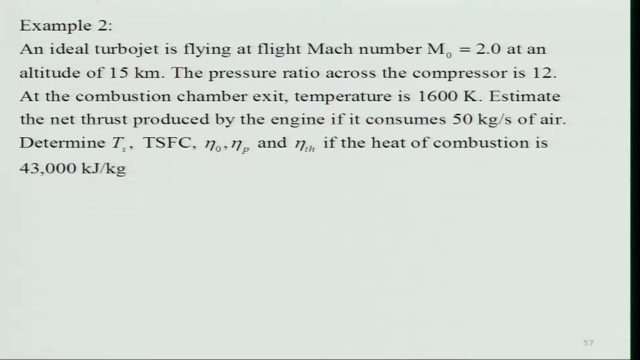 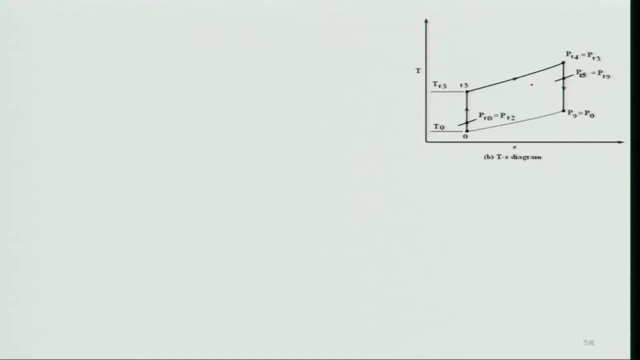 very easily. the flight mach number, sorry, flight velocity, that is v naught- is equal to root over gamma r t naught. t naught is given to you and gamma, you know, 1.4 r is 287, that is the specific, you know. gas constant: 287. for air it is 287.. And temperature: we have already. 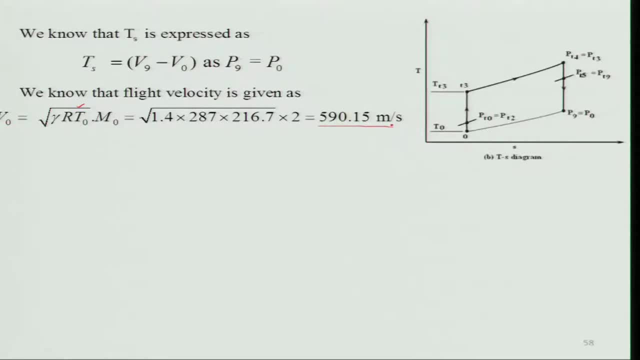 seen that thing- and you will get 590.15 meter per second. whenever you substitute these values, you will get this, which is quite you know higher. and this, if you look at the most of the turbo jet engine is basically used for the high speed or high velocity application. 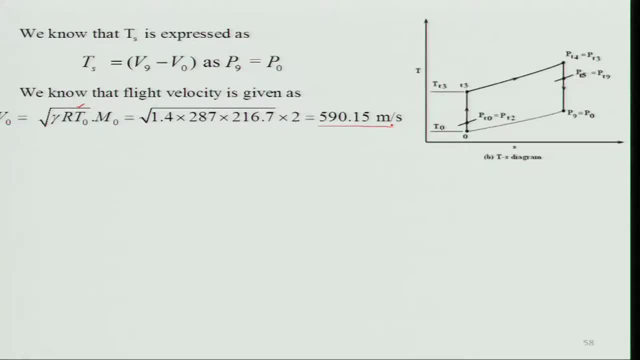 like fighter aircrafts and all thing right. So therefore the it can operate at higher flight velocity. so, but the nozzle exit velocity is to be determined because we are interested the finding out T, s and v 9 is a nozzle exit velocity. 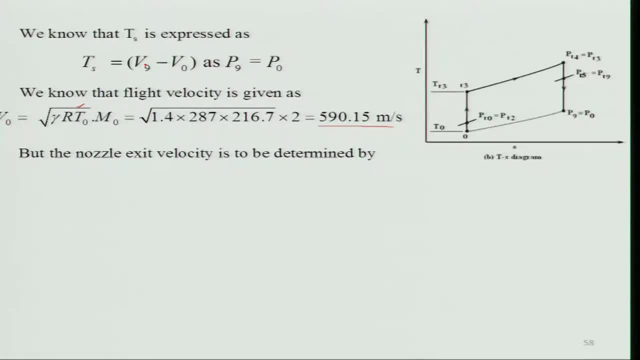 So that is the you will get, which is quite, you know, higher, and this if you look at the velocity. So we need to find out that. So if we need to find out that, so basically we can write down: V 9 is equal to root over 2 C, p, T, t 5 minus T 9.. So do we know really? 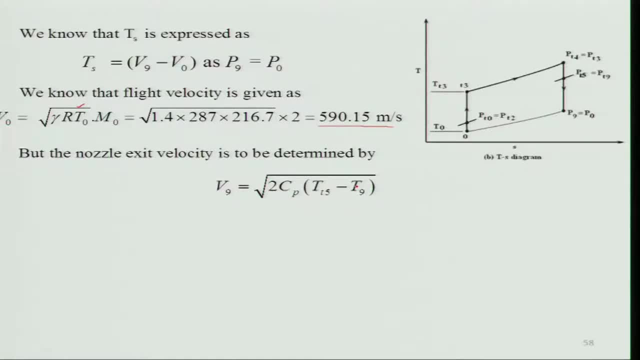 T 9, or is it same as that of the T naught? T 9 is here? certainly it is not, because it is, you know, not in the same place in the T s diagram. That is, of course, mechanically you can think of. other one is that it can never be, because you are adding heat and you 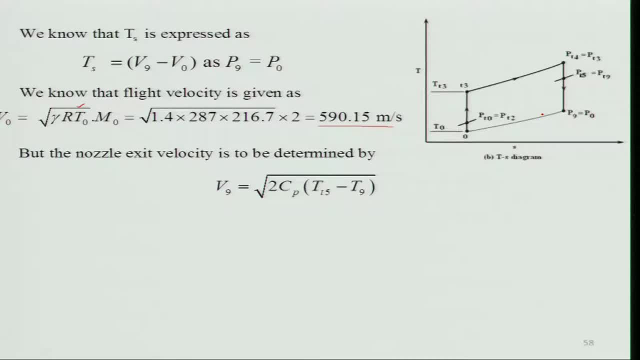 are of course expanding in the nozzle right. still the temperature will be higher than the ambient temperature. So we do not know T 9 and do we know this T t 5? why I have written T t 5? because T t 5 is equal to T t 9, right, in principle it could have been T t 9 by definition. 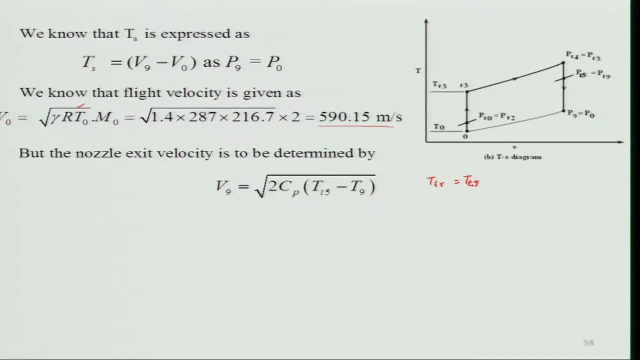 V 9 is equal to root over 2 C p, T t 9.. T t 9 means total temperature at the station 9 is that clear. but we do not know T t 5, but of course I know this. T t 4. T t 4 is what is given as 1600 Kelvin. but I know this. 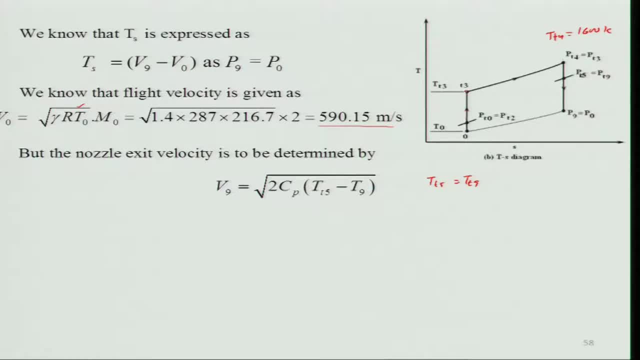 temperature T naught right here, but I do not know what is this temperature T t 3.. If I know this T t 3, then you know, I can, you know, I can find out what will be the pressure here. So from this here I can find out how much expansion is taking place in the turbine, because 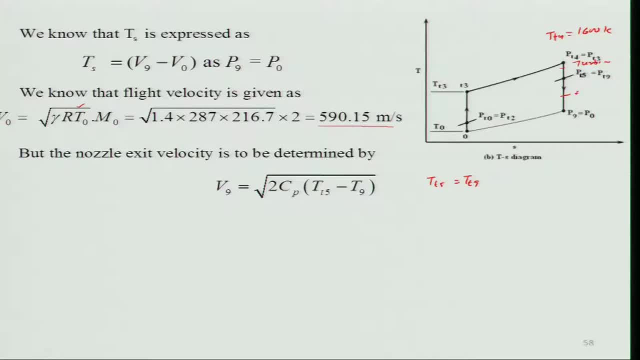 this is turbine expansion, right, and this is your nozzle. So I do not know. I can start from here and do that, but I need to know also the pressure. therefore, I will have to go in a systematic way. So let us look at how I will do that. So, in order to evaluate, 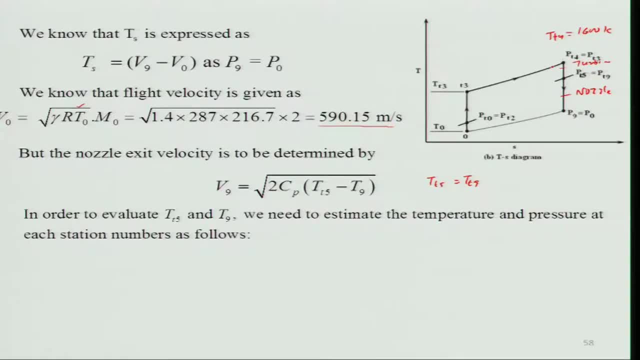 T, t 5 and T 9. we need to estimate temperature pressure at each station. numbers right, So I will do that because at each point I need to know the temperature and pressure. Sometimes you can avoid, particularly for an ideal cycle, but, however, in real cycle you will have to. 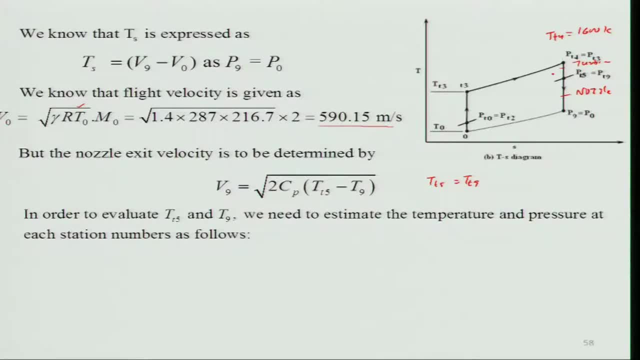 go through the same systematic procedure, otherwise you cannot really handle it. Of course, some of you can use your intelligence to do that. that is a different thing, but it is better to follow a systematic way. So let us look at air intake, what is happening? total pressure and temperature. that is total. 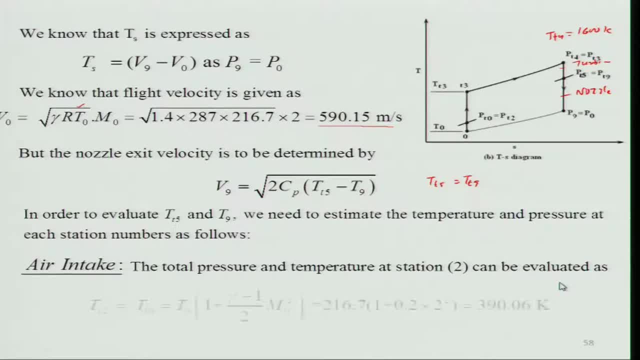 temperature station 2.. This is evaluated very easily, right? So we know that T t 2 is equal to T t naught, right? that means in the air intake there is no heat transfer or it is adiabatic process. So therefore, 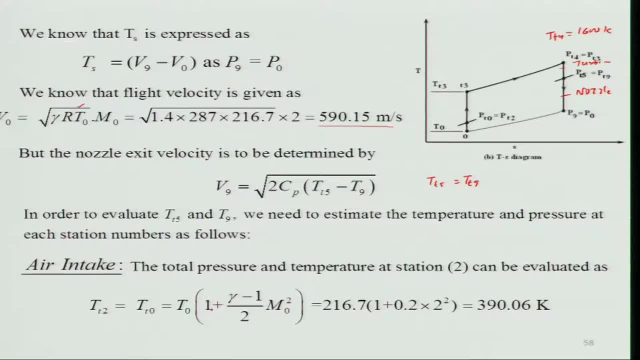 T t 2 is equal to T t naught, which is nothing but T naught plus 1 plus gamma minus 1, divided by 2 m naught square. So m naught is given to you, gamma is not given and this is given. 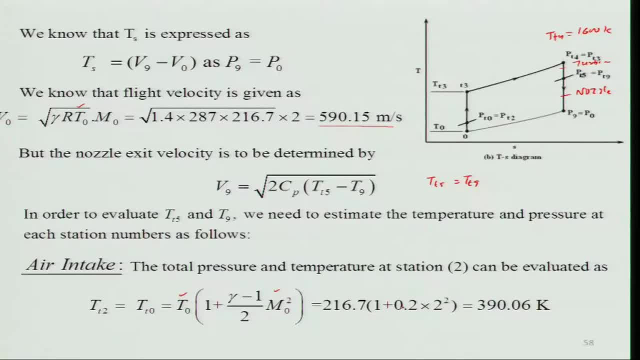 So you can find out 390.06 when you substitute this value right And you can see that it has increased from 216.7 Kelvin to 390, because the Mach number is 2 right, which is higher. If it is Mach number is small, then this will be not really. 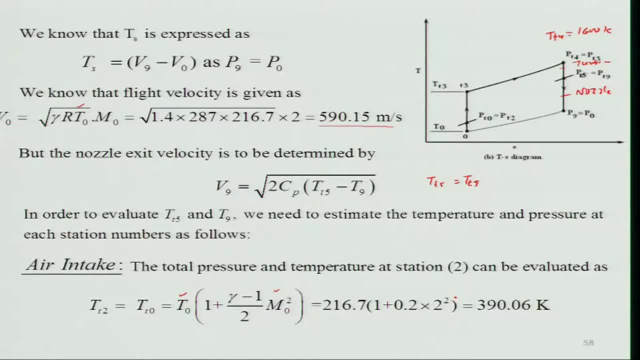 varying. for example, you know, if it is Mach number 0.5 or 0.2 or 0.3, then this, you know, static temperature T naught will be almost similar to the T t naught, So that you should appreciate. 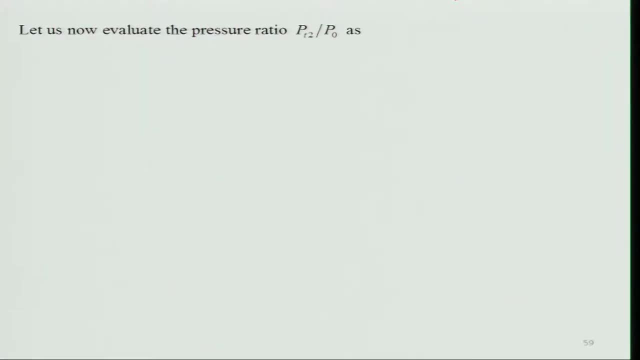 to now evaluate the pressure ratio p t 2 by p naught, which is again, will be using isentropic process, because at ideal cycle we are considering. So p t naught is equal to p t 2. I mean like then I can t t naught by t naught and if you look at, we know this value and we can substitute.